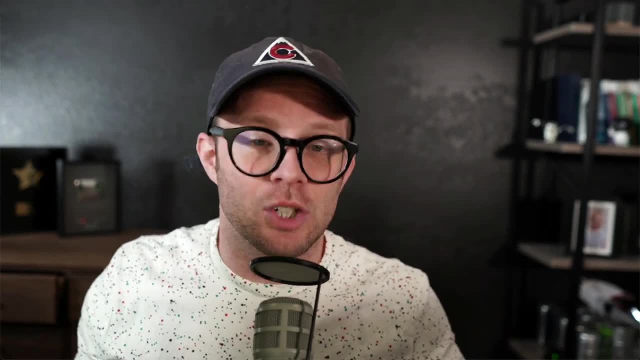 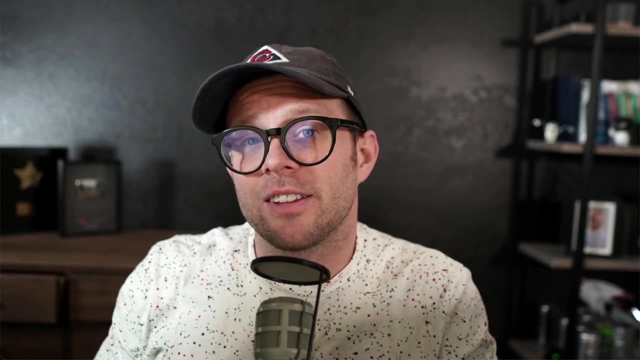 components. we have other frameworks that are on top of things like a virtual DOM, like react and view. then you have things like Svelte that use just the DOM, And then you have things like lit that are basically a layer on top of web components. Now, if you don't know what web 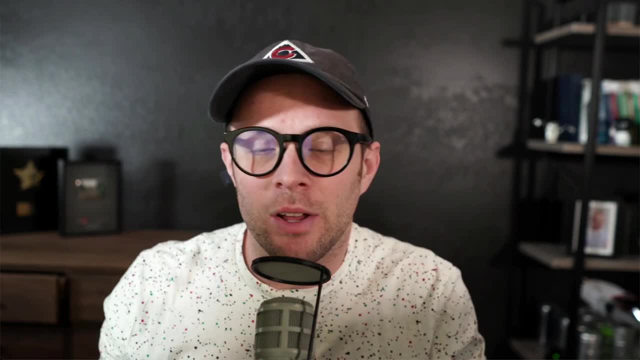 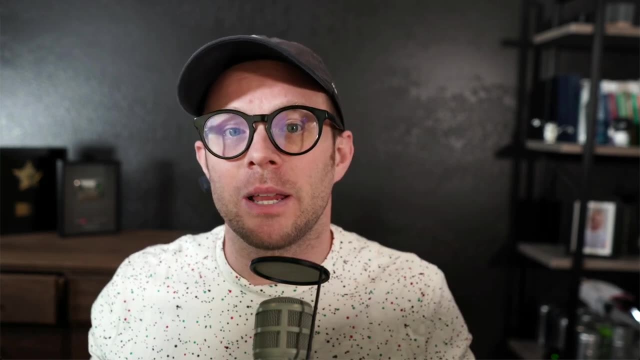 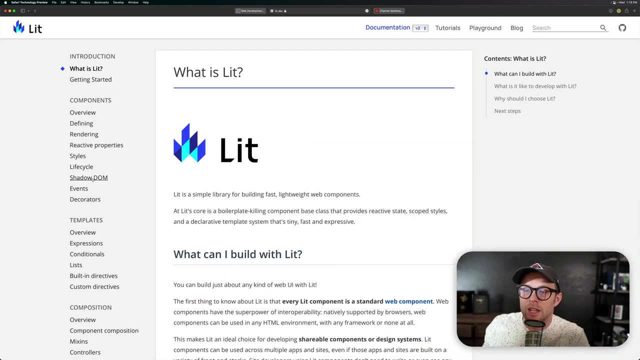 components are. we have a whole what is? video on web components as well, But the quick explanation about web components is it's components in the browser, using only browser APIs. Now, that's a very simplified way of explaining them, considering there's things like the shadow DOM and explanations there. However, 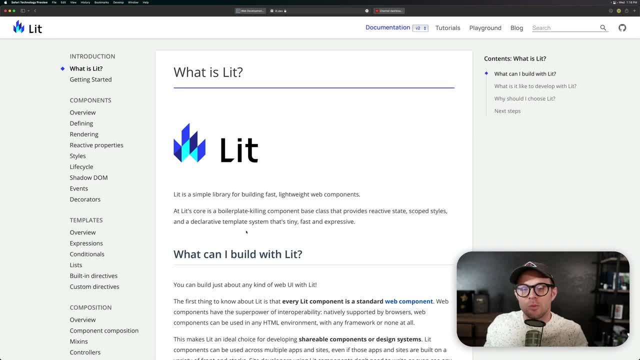 basically, web components are a way to build components in the web using only browser APIs. Now, why would you want to use lit then, if browser APIs allow you to build web components? Well, the syntax for working with web components is not always the best, And it's not always easy, And especially if you're coming from react. 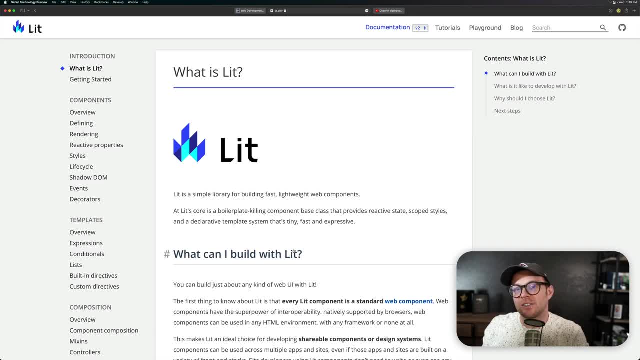 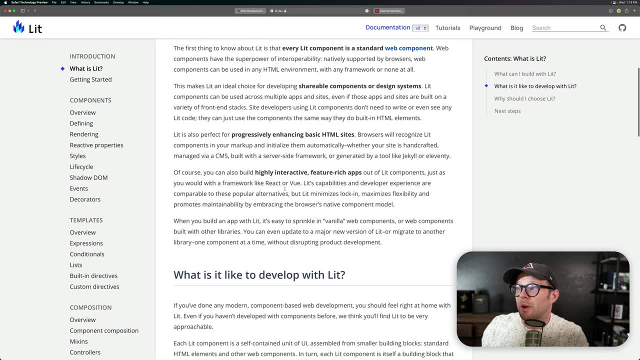 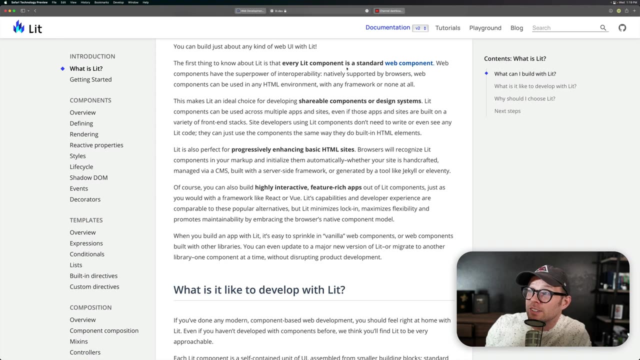 view. Svelte or Angular coming to web components can feel like taking a giant step backwards. So in comes a library like lit that gives you the ability to have interactive, feature rich apps, progressively enhanced basic HTML sites, shareable components or design systems. 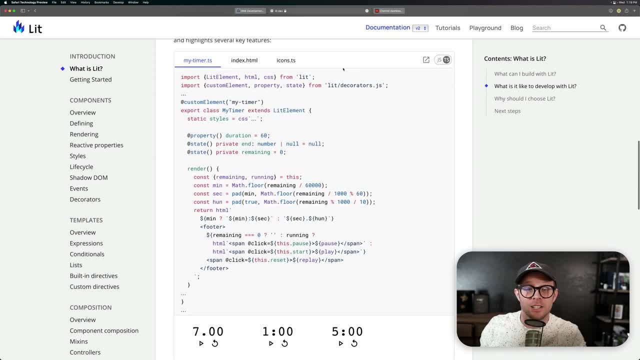 but on top of web components. Now, if we want to take a look at some of the syntax, this is largely what it looks like. you'll recognize some things as being JSX, like where we have a template literal, template tag literal, to do our. 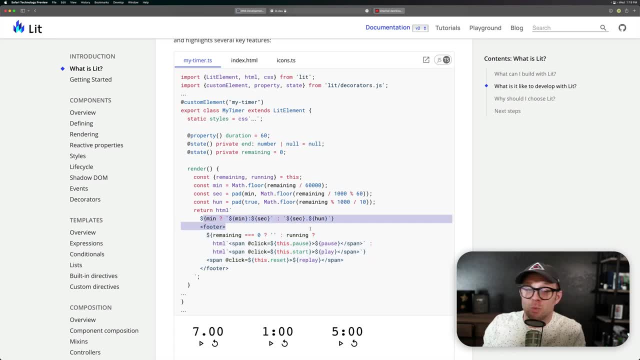 templates, our HTML templates. we're using actual JavaScript string interpolation in here, So nothing fancy right, It's just string interpolation inside of a backtick function, And then we have a render function just like you might have within a react application. So at the 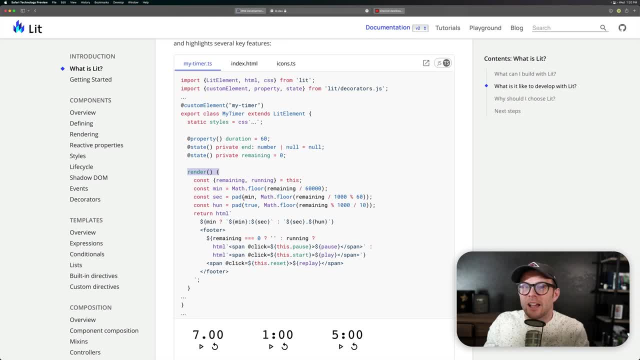 end of the day, what you end up having is something that feels almost like a class based react component, but it's also using things like decorators, as you see here, to do things like local state as well as props. So props are properties and you define them with. 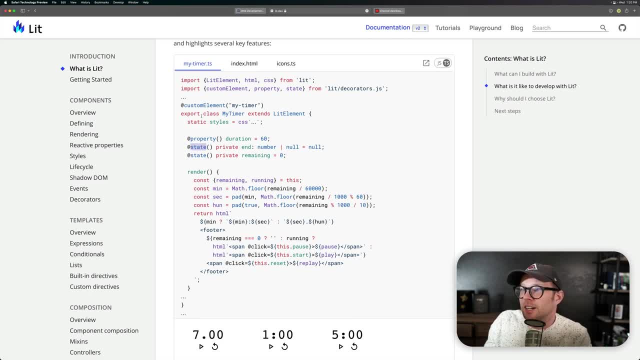 a decorator state you define with a decorator. you can do static CSS with a static property inside of this class And components are all based on a class. Now the custom element directive allows you to name and define a class, So you can define a class. you can define a class you can. 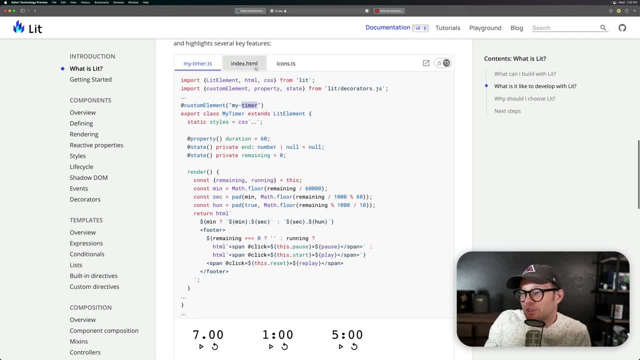 define a component. Now, this syntax is interesting. it is kind of a mashup of many things, In fact. I think maybe people from Angular might look at this the most. you know most find it to be the most normal. maybe, if you're coming from this, from a react class based component thing, this would 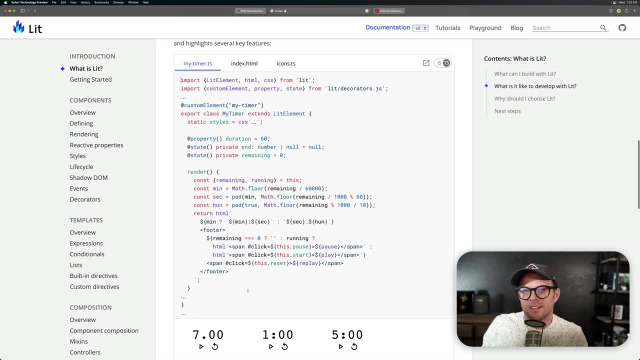 look kind of normal to you as well. Me personally the syntax is fine. It does feel a little bit tough to read at points, But I think I'm sure once you get used to it you'll be able to read it. So 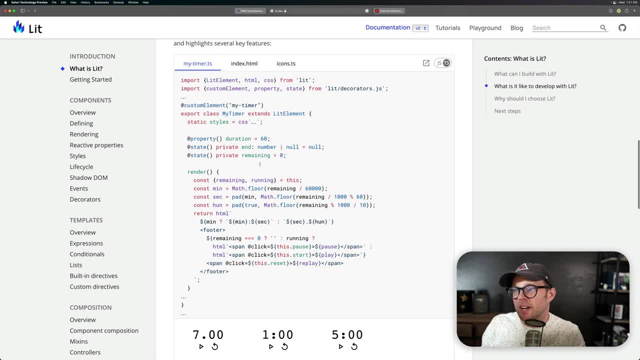 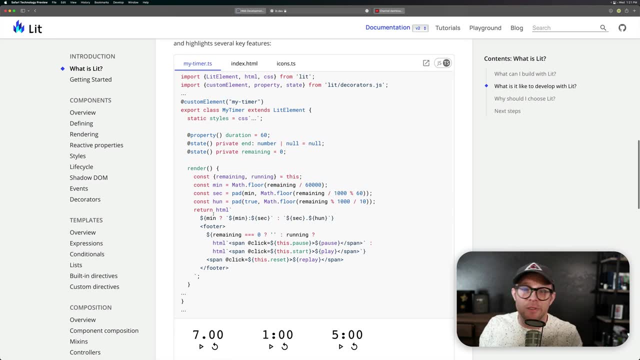 it's fine Either way. the reason why lit is so great is because it allows you to do things like this: creating a timer based application and much less code than writing straight up web components, which I've done and personally don't love. I love web components, I love the idea of web. 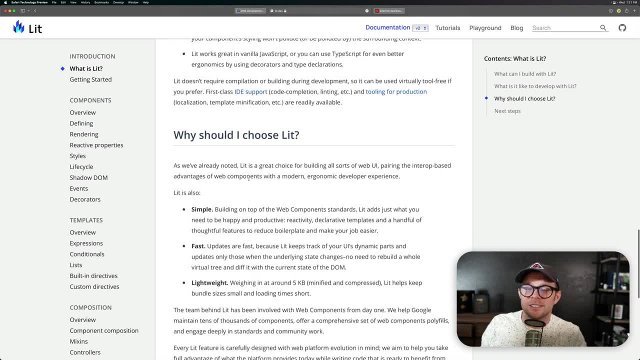 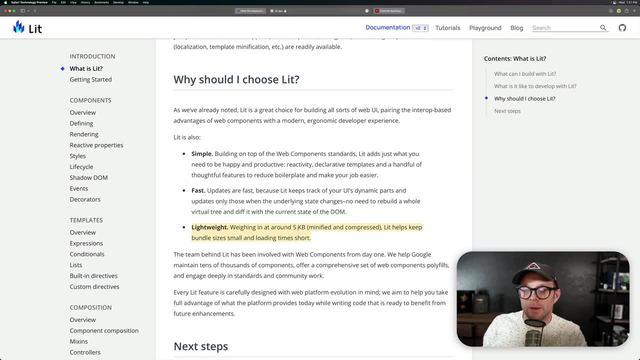 components, But I've always found that the syntax to be not a lot of fun to work in, So why should you choose lit? It is simple, fast and lightweight. It only costs around five kilobytes minimized or minified and compressed. So 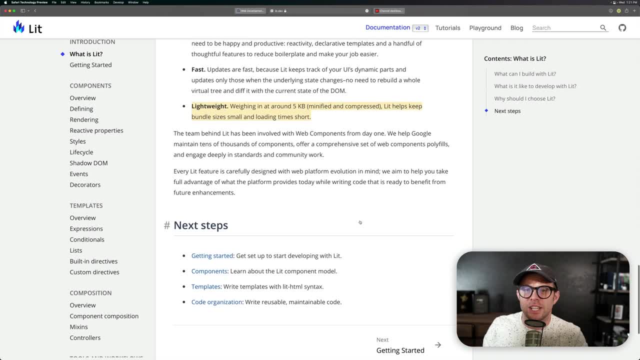 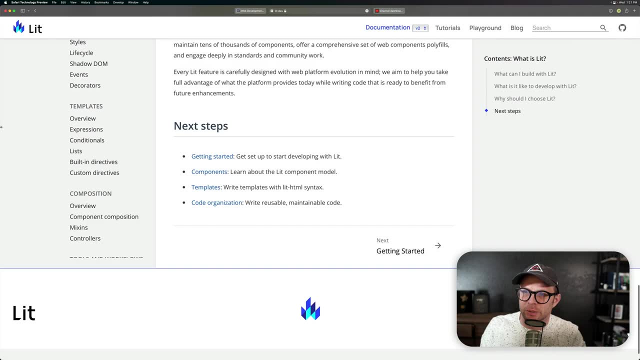 it keeps it nice and small. It's always a good feature, especially in this modern world where we're shipping a ton of JavaScript. The last thing you want to do is ship a big old library with anything you're doing. Now there's a lot more here in lit, But if we're giving a high level, 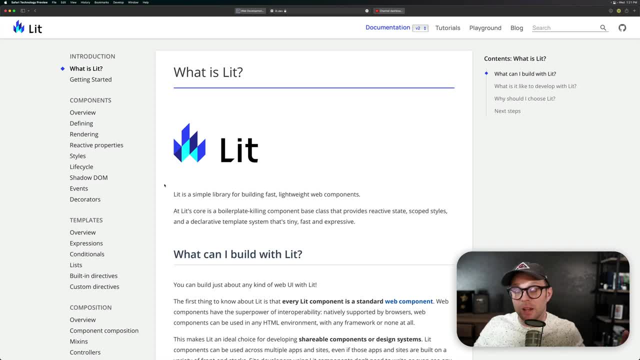 view of what the heck lit is. at a big, broad viewpoint, lit is a library that sits on top of web components to allow you to build components for the web using web components, but a better structure, more unified, more structured syntax. A common complaint you'll see with web components. 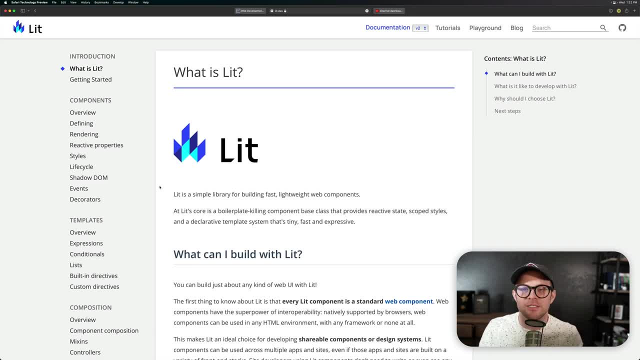 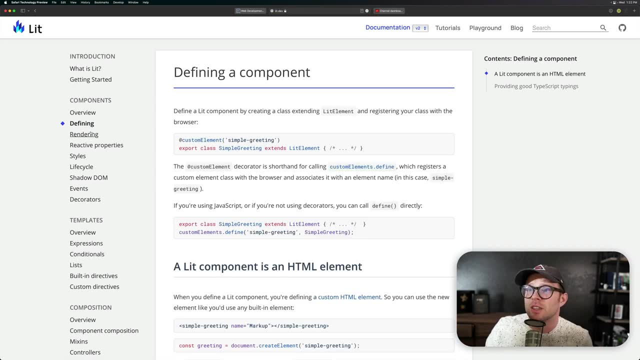 is that when you look up how to do anything in web components, there's 10 different approaches because there's a lot of different ways to do it. But with something like lit, you have a little bit more conventions on how to do things And again it's all class based. you have things like